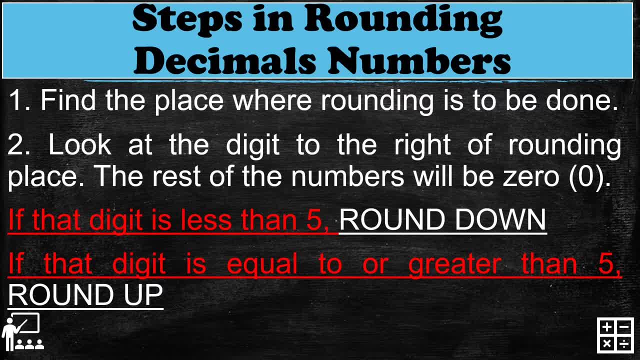 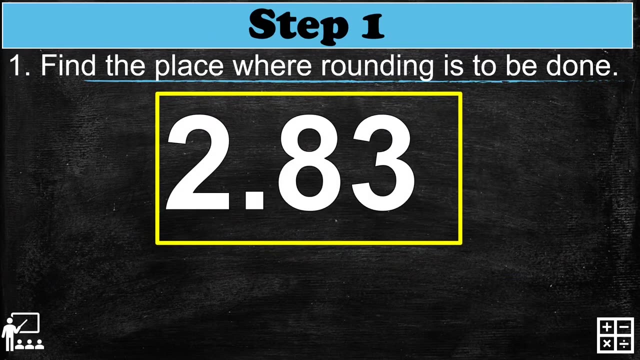 Round downs means we're just going to remain the number as is, And if that digit is equal to or greater than five, we're just going to round up. Round up means we're just going to add one. Let's try. So I have here 2.83 or 2 and 83 hundredths. 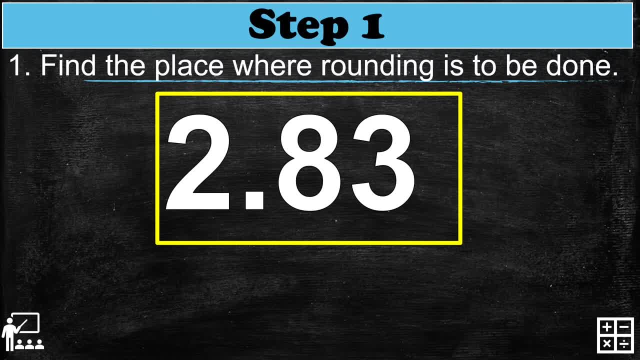 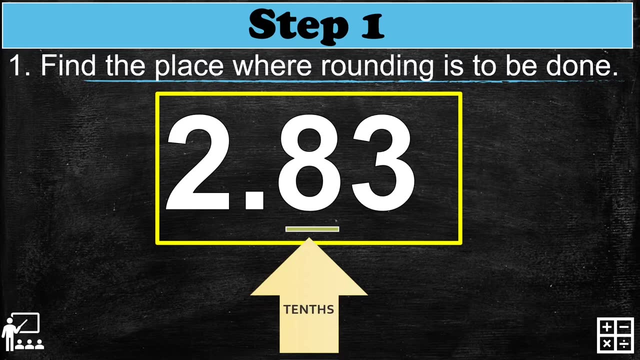 So first step is to find the place where rounding is to be done. A while ago I said we're just going to focus on the tenths place And number eight is our tenths place digit. Step two: Look at the digit to the right of the rounding place. 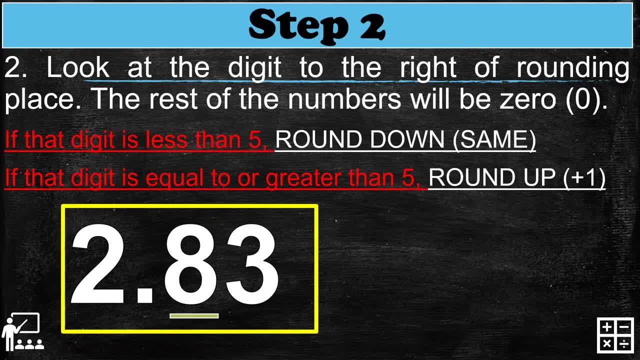 So again, the eight is on the tenths place And the number to the right is number three, And three is less than five. And if that digit is less than five, we're just going to round down. It means, if we're just going to stay, the number eight. 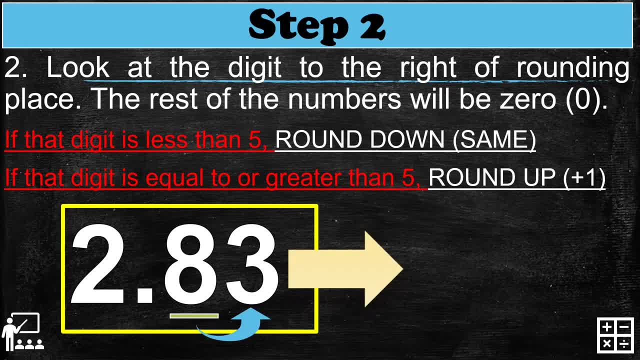 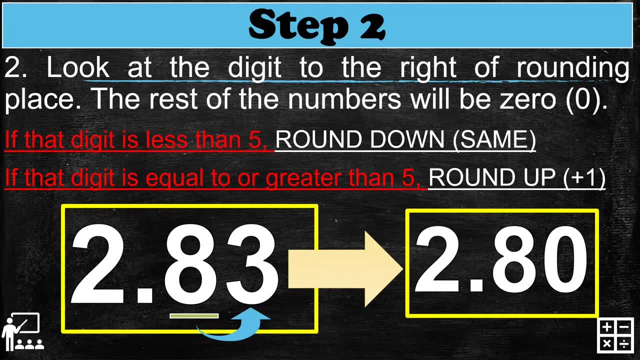 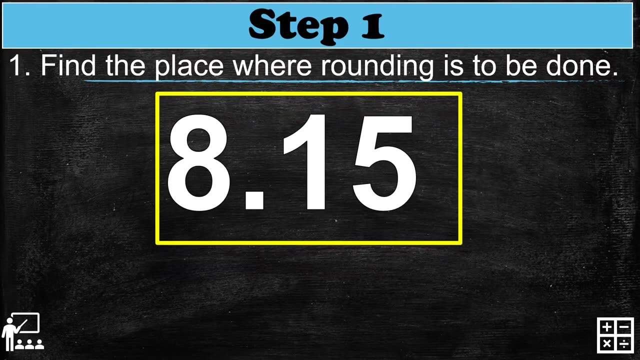 So that the rounding of 2.83 is 2.80. And the rest of the numbers will be zero. Three becomes zero. Take a look at my example number two. I have here 8.15 or eight and 15 hundredths. 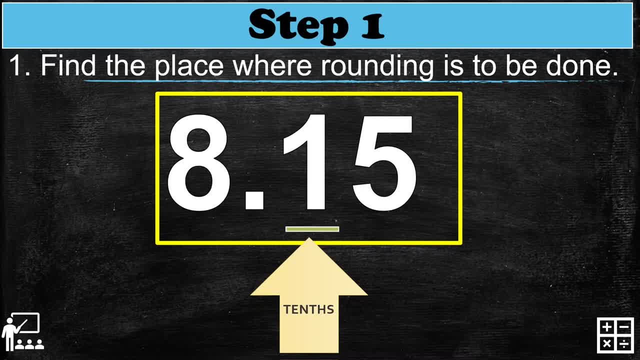 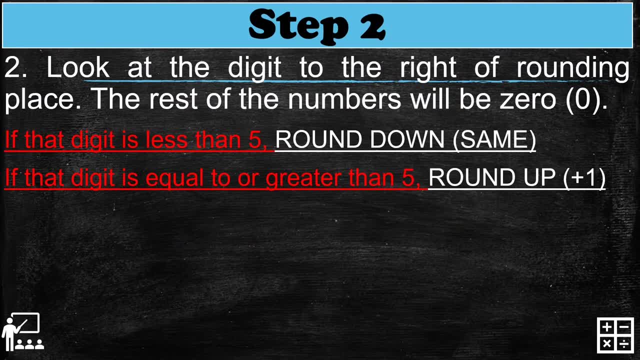 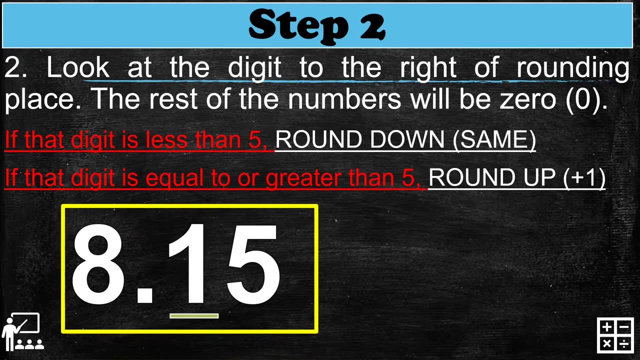 So again, we're just going to look at the tenths place value digits, which is one. Step two: Look at the right to the, look at the digit to the right of rounding place. So the number to the right of the rounding place is number five. 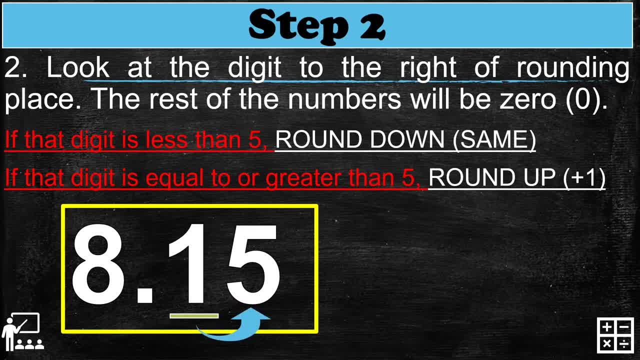 And number five is equal to five, So that we're just going to round up. Round up it means that we're just going to add one to the rounding number, which is one. So one plus one, it will give you a two. 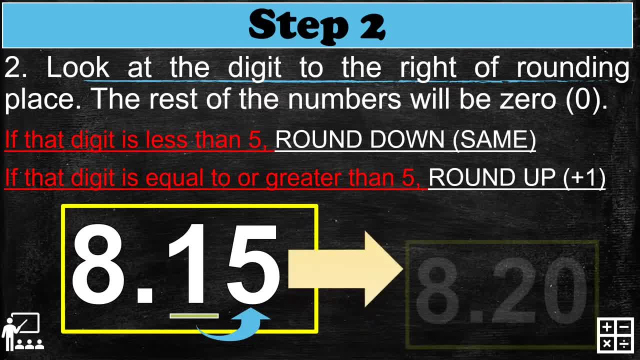 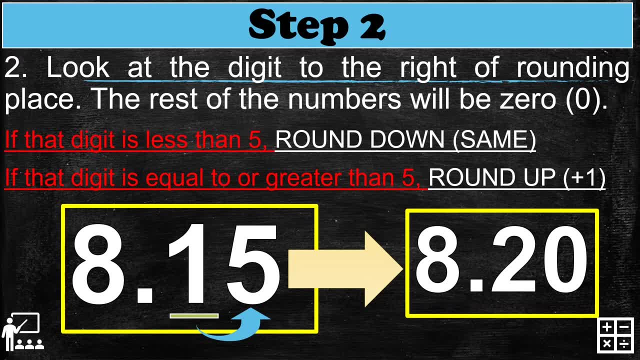 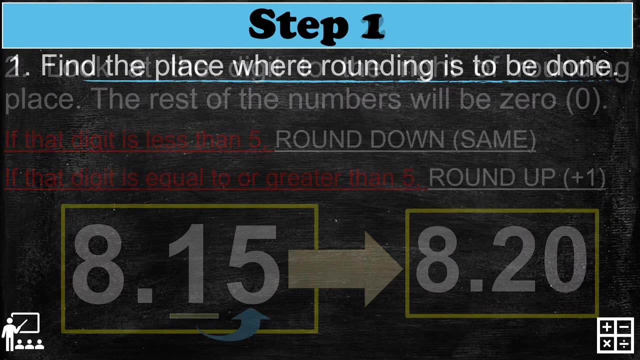 So our new number is, our new decimal is 8.20.. It become number two because it equal to number five. And if it is equal to number five, we're just going to round up or just add one Again. another example: 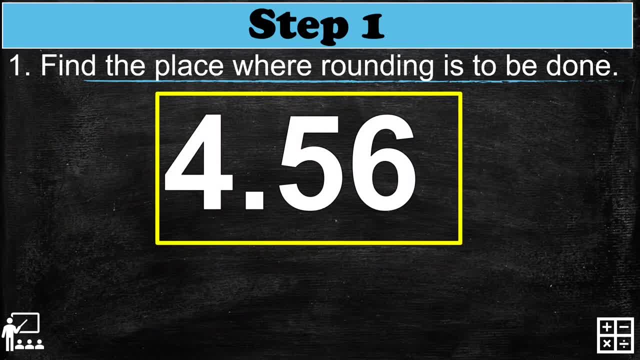 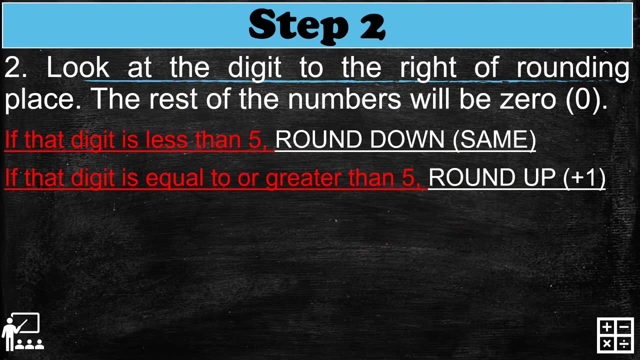 Four and 56 hundredths. So again, find the place where rounding is to be done, And we're just going to focus on that, We're just going to focus on the tenths place, which is five, And again, we're just going to look at the right of the rounding place. 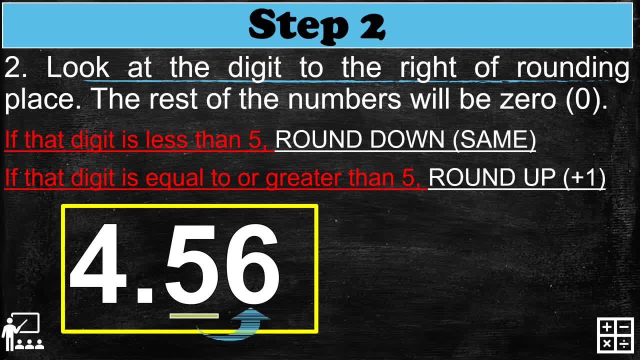 And the number to the right of the rounding place is six, And six is greater than five. And if that digit is greater than five, round up Again. round up: it means that we're just going to add one to the rounding number. 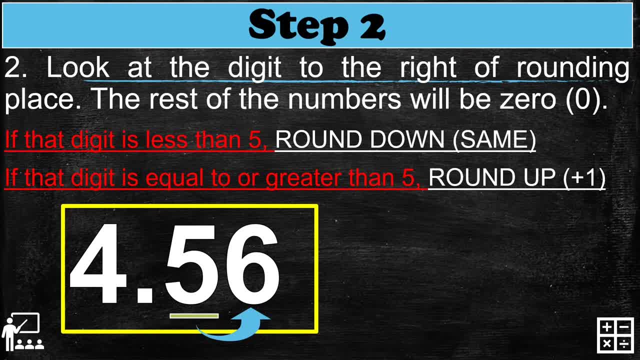 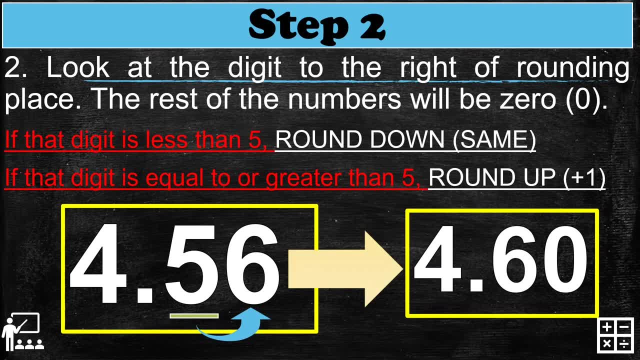 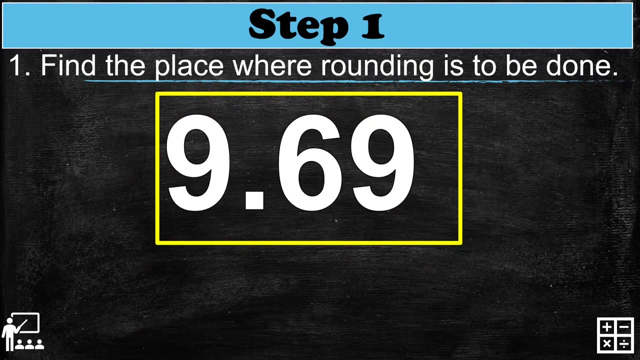 So four point four and 56 hundredths, it become four and 60 hundredths. We just add plus plus one, It will give you a six And the rest will be zero. Another example: Nine point sixty, nine or nine and sixty, nine hundredths. 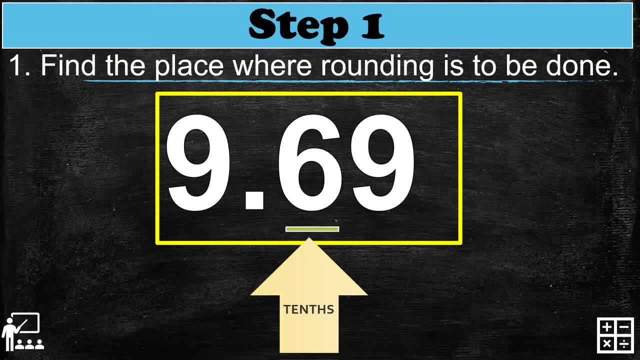 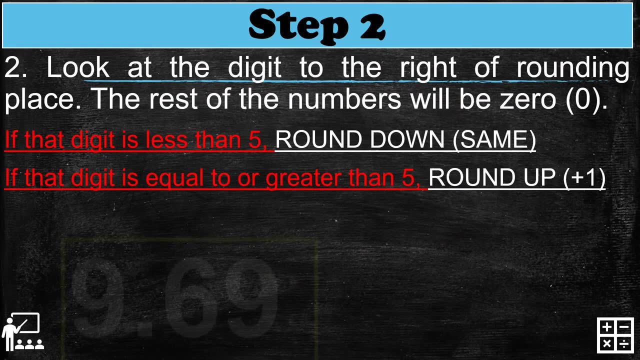 So again, we're just going to focus on the tenths place value And our number to the tenths place value is number six And step two. look at the digit to the right of the rounding place And the number to the right is number nine. 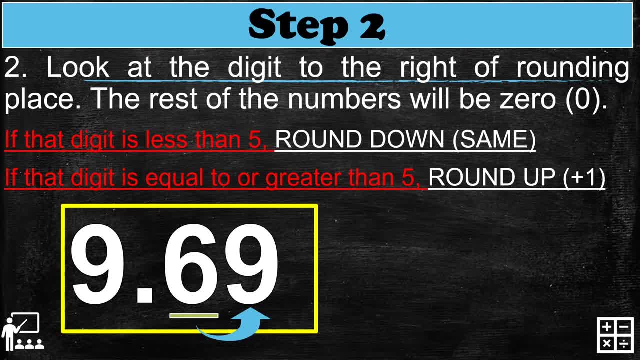 And number nine is less than or greater than five. Okay, it's greater than five. So that we're just going to round up Or we're just going to add one to the number six. So six plus one, it will give you a seven. 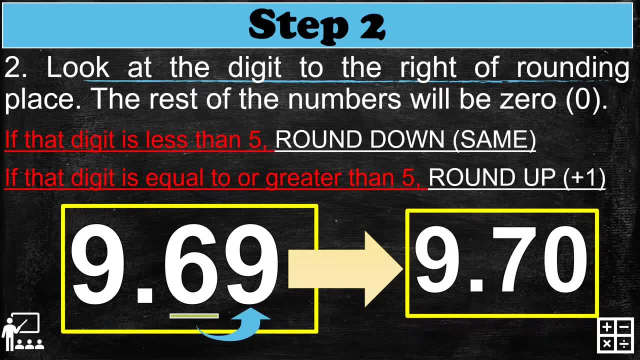 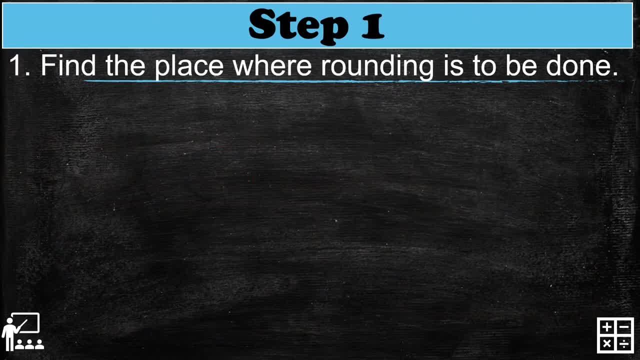 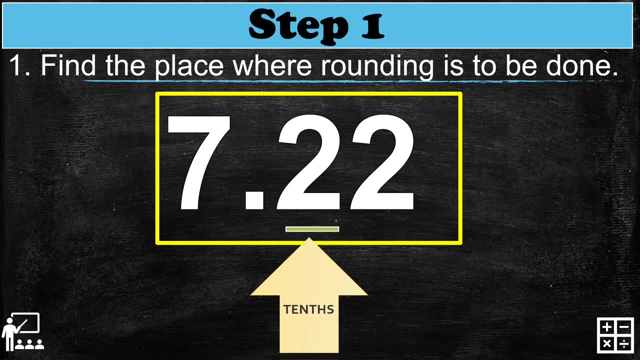 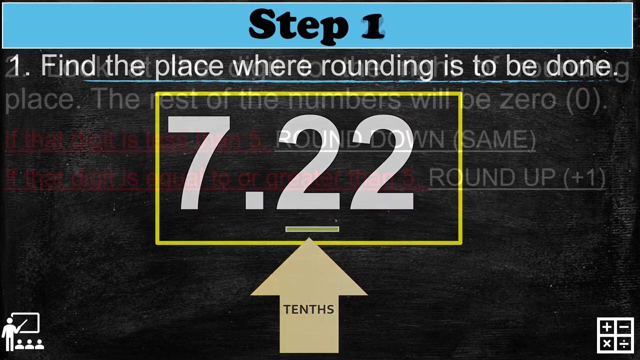 So our new decimal is nine And seventy hundredths, Another seven and twenty two hundredths. So the number to the of the And the number which is located of the tenths place value is two. And second, or step two, is to look at the digit to the right. 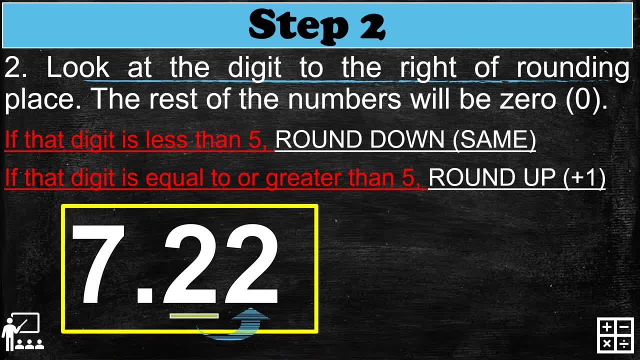 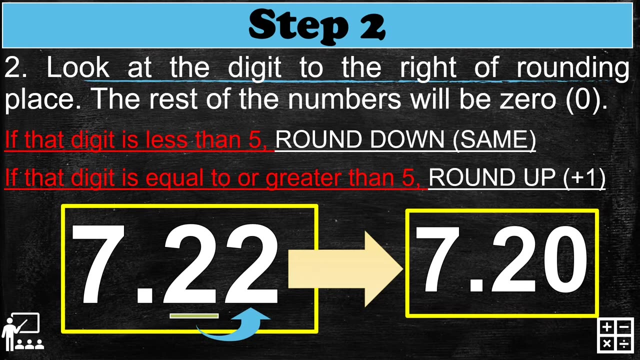 So the number to the right is two, And two is less than five. So we're just going to round down. Just remain the number which is two, And our new number is seven point twenty, Number seven and twenty hundredths, And the rest will be zero. 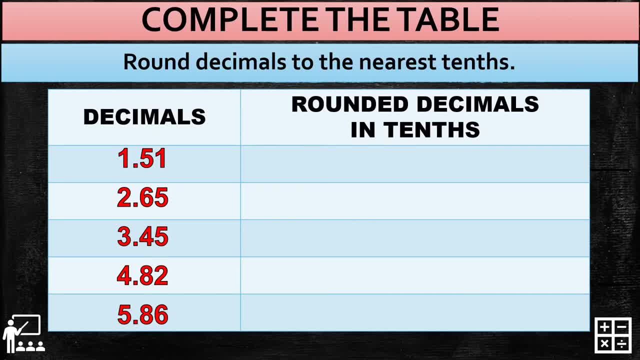 Okay, let's try. So I have here one and fifty one hundredths, Two and sixty five hundredths, Three and forty five hundredths, Four and eighty two hundredths And five point five and eighty six hundredths. Okay, let's continue. rounded decimals in tenths. 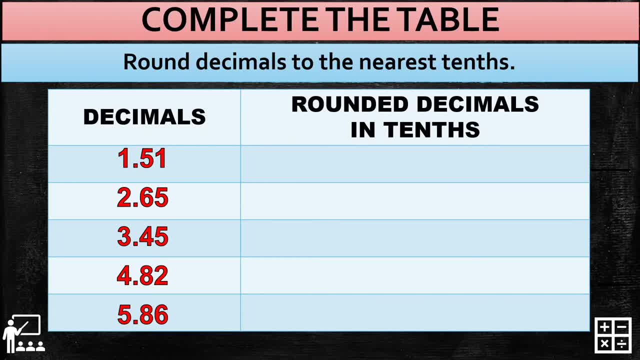 Just like we did a while ago, I'll give you twenty seconds to answer for this activity. Just round: decimal to the nearest tenths. Reminder: the tenths is located after the decimal point. Okay, your twenty seconds starts now. Ten seconds. 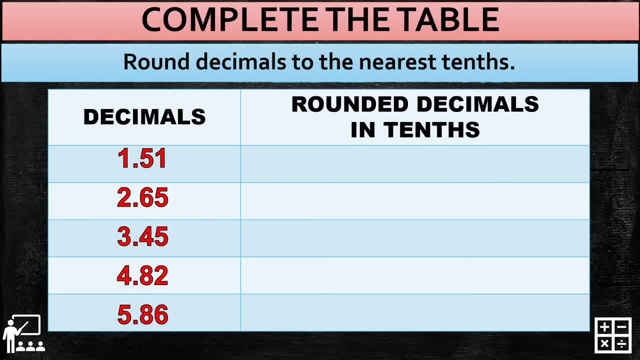 Five seconds Time is up Again. I will show you my answer and compare with your answer. So number one: One and fifty one tenths. It become one and fifty cents Because the digits on the right of the five is one.